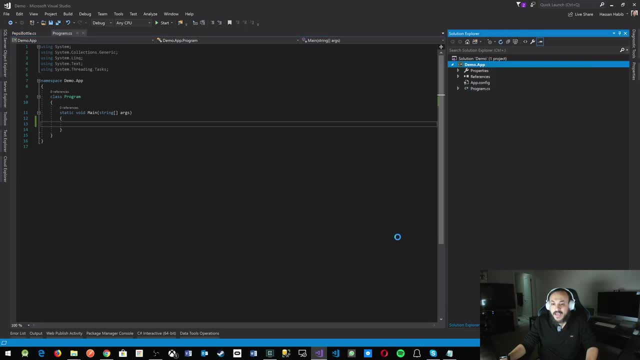 What's that memento pattern? Let's go ahead and create a new class And let's say that class is called student And let's give that student some properties, So let's say string status, So that's a student that has a status. 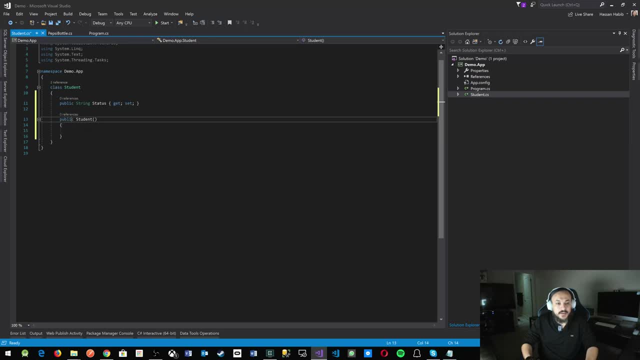 And let's have a constructor in here that takes in that instantiates this status to pending approval, Like this, Like that, Right. And then there's another function that we want to build. There's a function we want to build that says start admittal admission process. 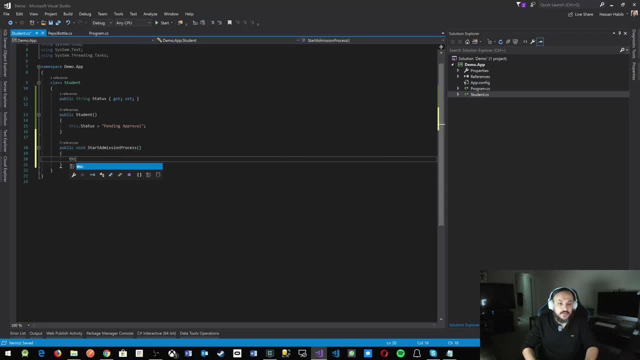 So before you start the admission process, you're stamping your data, which is the student in that case with admitted Right. The problem with that is if something blows up and let's go give you an example here, Let's say I created that student in here. 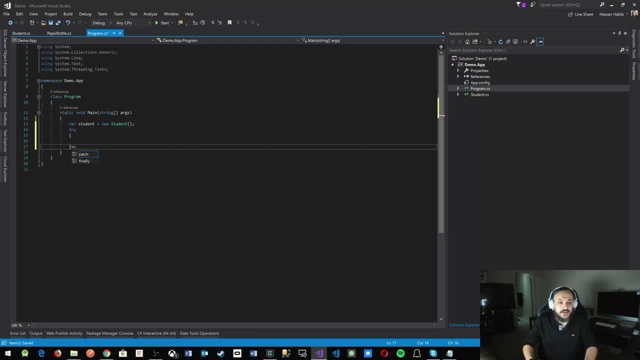 And then let's say I have a try catch block in here And that just will resemble a fake error that happened. I don't even need that, I could just go like that. And let's say, you know, just console. 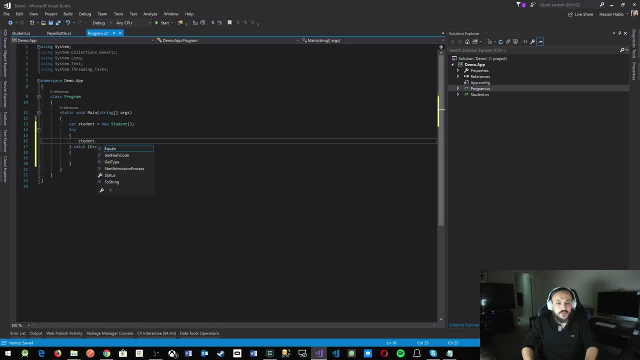 We throw any exception- It doesn't matter- in here. And let's say, when I'm doing this start admission process, something blew up. So I'm going to throw an exception in here and say: something blew up while I'm doing the start admission process. 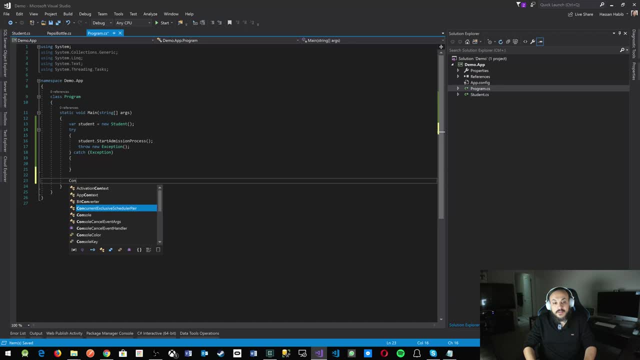 The problem here is that the student status- student status after failure- will be admitted, which is not what we want. Console, We don't want. we don't want the student to be on admitted status, because that means we're having inconsistency of data. 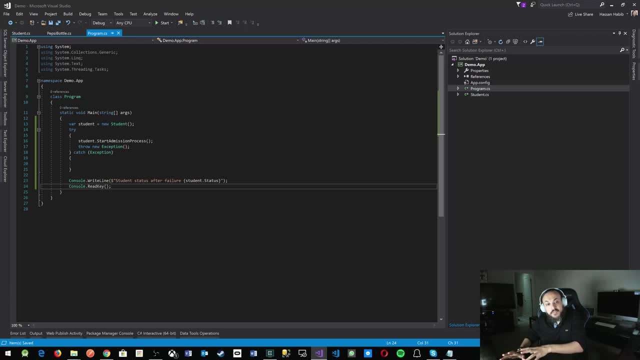 And we need somehow to find a way to revert that student object back in time to the point where it was before starting this new operation. This is very high defensive programming, especially when you're working with with RESTful services. They are stateless. 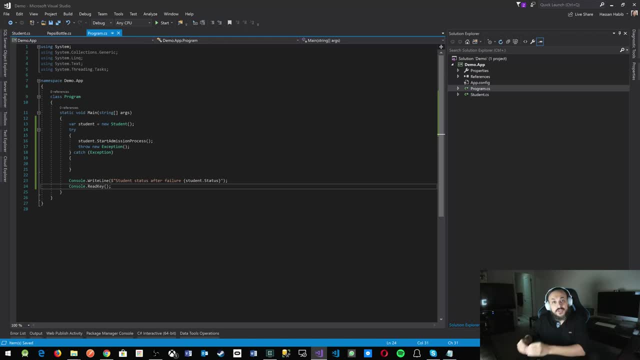 You know you want to make sure that your current local state for your data makes sense. So let's, let's, let's put another, another, another line in here that says: here's the student status before, after processing. 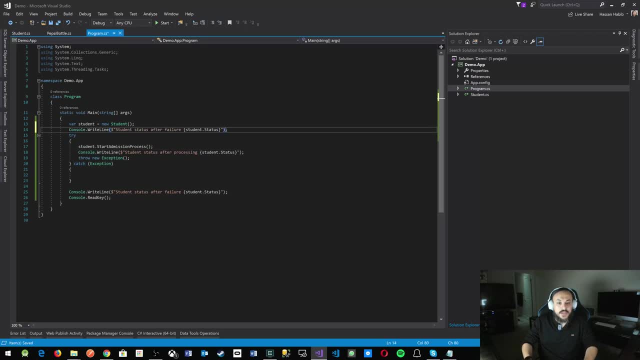 or attempting to process, right, And let's throw one in here that says initial student status. And that's what we want: Initial student status, Right? So if I run my application now, things will blow up. I'll say it was pending approval. 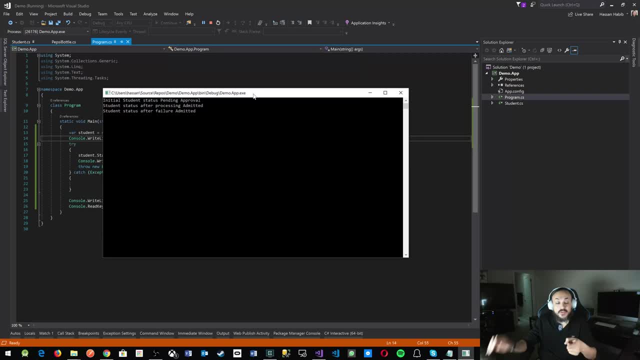 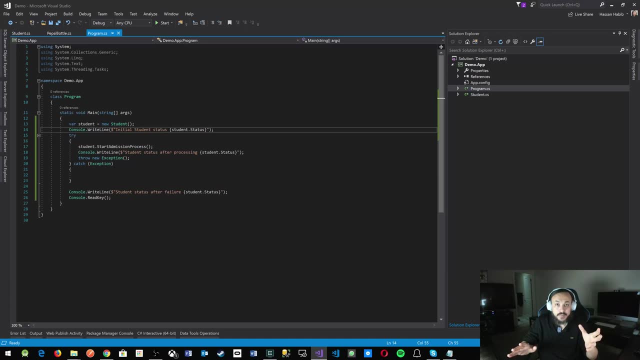 started processing admitted, but after the failure the student is also admitted. Imagine if your student object has like 20 properties across the entire object. I would question why you have an object with 20 processes with 20 properties. but let's just assume right. 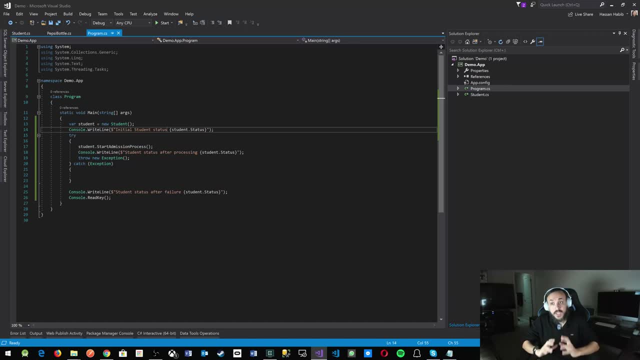 And you want to revert over all of that. It'll be very hard. It'll require a lot of data fixing. You need to go back and fix that data and make sure that everything is in place and you have to write scripts and it's a complete waste of time. 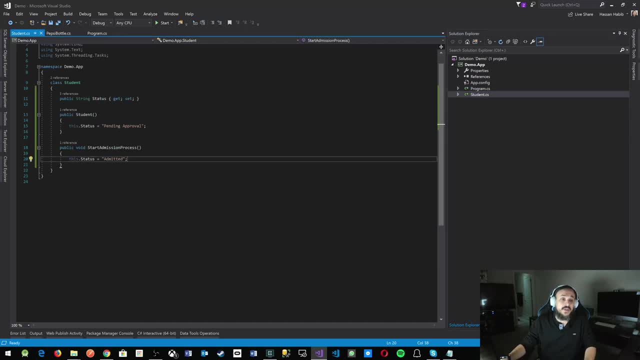 Instead, you could implement the memento pattern, And I'm going to show you how to do that. We could build a class in here that call it memento, And what this class has, it will instantiate itself by the same properties that your object that you want to revert back has. 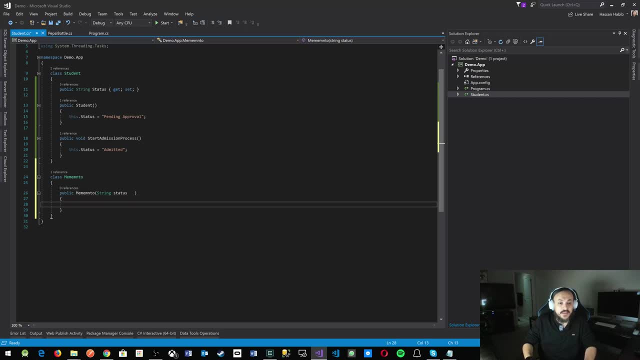 So you could say string status. that's what you get and you have a. let's throw a read only, string read only. let's say read only public, read only, string status, status like that, and what sitters or gears on that? these are read only and we go and say thisstatus. 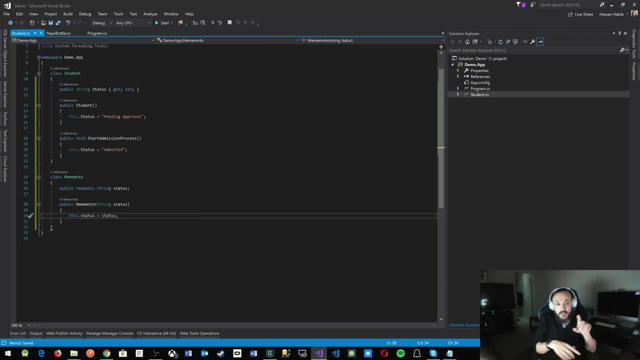 equals status, whatever we're passing. So you're passing in the same values that you want to be able to revert, right. But then back in here, we want to do that little modification. we want to instantiate a memento. what did I write? not memento, it's memento. let's do that memento, I think. 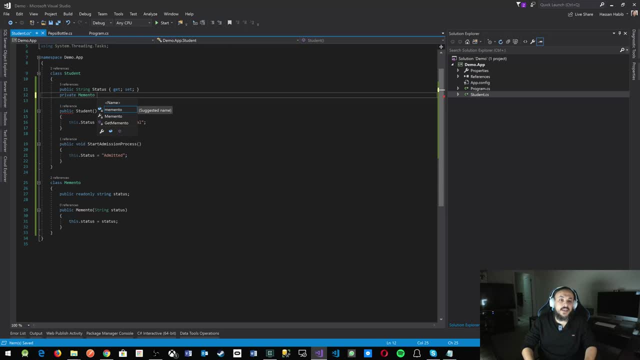 that's what it's called. and let's say memento. Let's just call it memento, right? And when we're instantiating that student object, we want to go and say, for that memento, let's instantiate with the same initial values that we had for the student, so we can revert back. 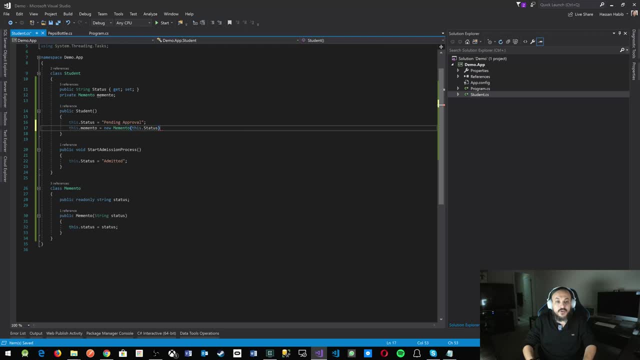 to that point. So let's pass in here and say thisstatus, So I'm basically passing it- its initial status, initial status to that memento pattern, and then I'm going to throw here a method that says revert. And what this method is going to do, it's going to say: go to that status and get that. 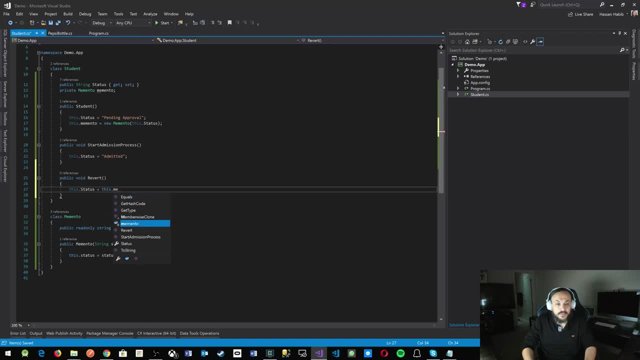 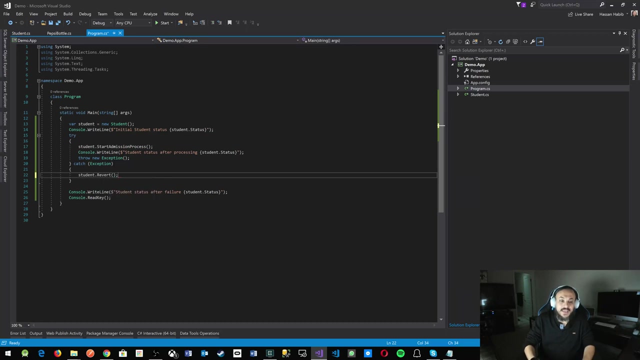 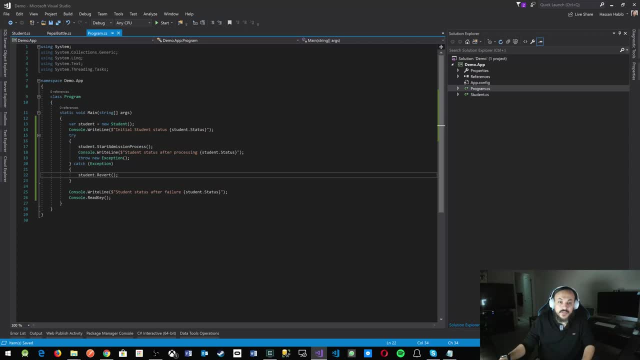 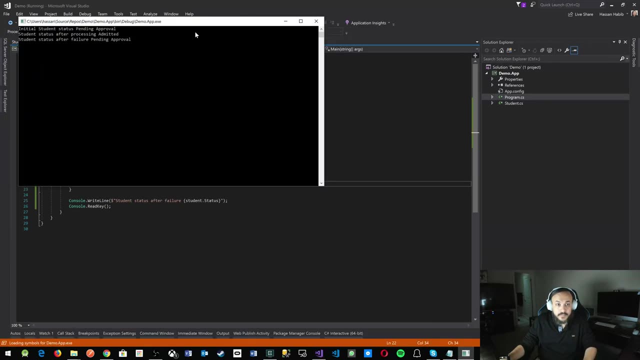 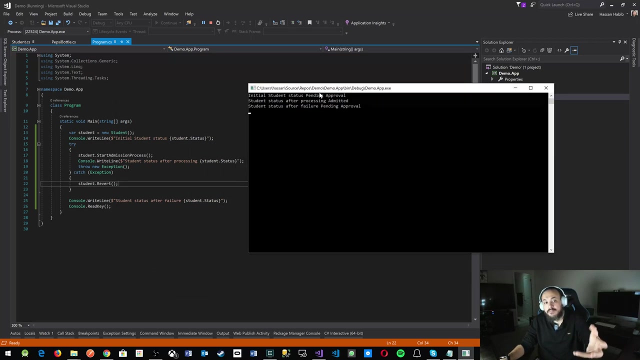 Now when we run, let's see: our hypothesis here is that this will be pending approval- admitted and then pending approval again. Is that the case? Let's see, There you go: Pending approval- initial state, start processing. something blew up. revert, put the status. 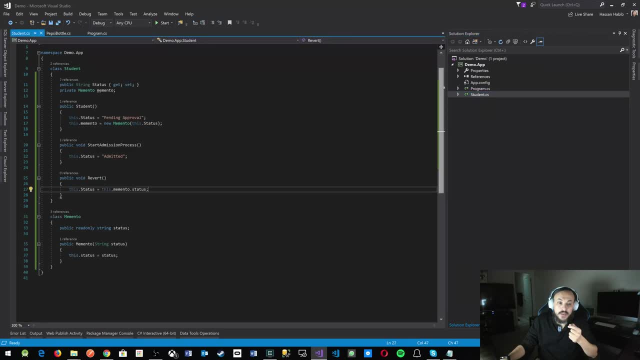 in there. you're good to go Now think about this for a while. So it has some storage concerns, especially if you choose to have reverse. I'm going to tell you that this is not going to work, So I'm going to say reverse. 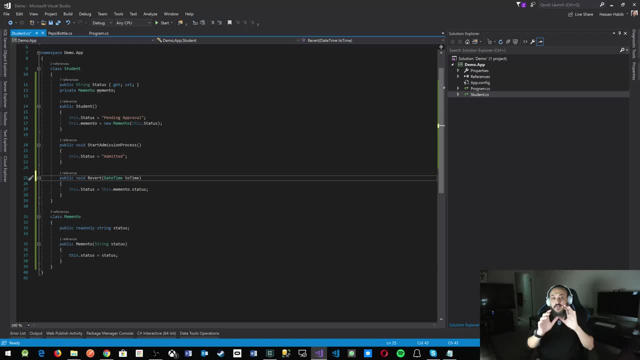 So I'm going to say reverse and then I'm going to say revert. It's going to say revert, give you this option of date time And you get to go back and say: revert, my object to a certain point in time. 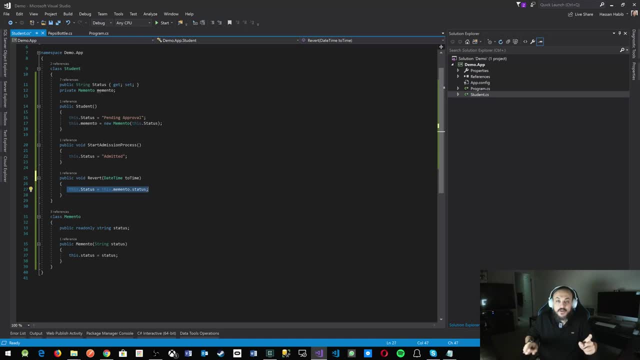 So you're going to have some sort of dictionary in here that goes and looks up of copies of that object and reverse it to a certain point. So don't use this model excessively, especially if you're going to use the entire document in a database.